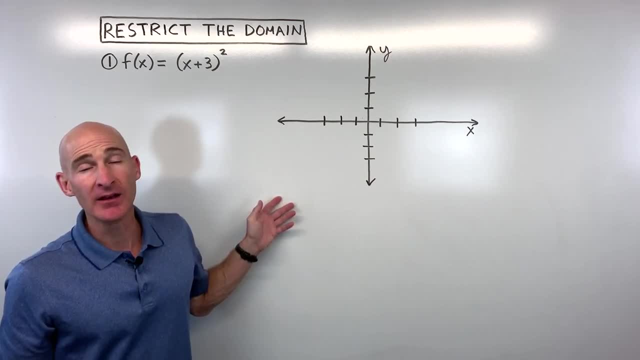 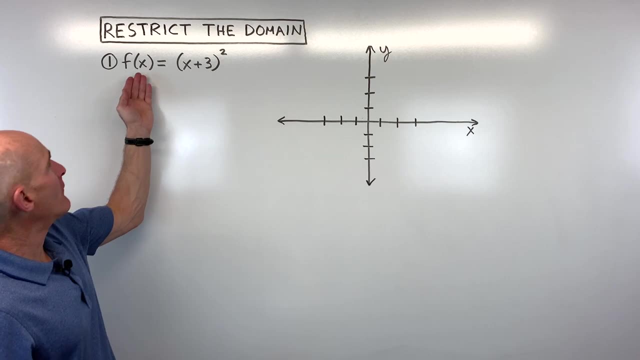 In this video you're going to learn how to restrict the domain so that the inverse is a function, And we're going to go through two examples together. So let's start with this first example. If we have, f of x is equal to the quantity x plus 3 squared. 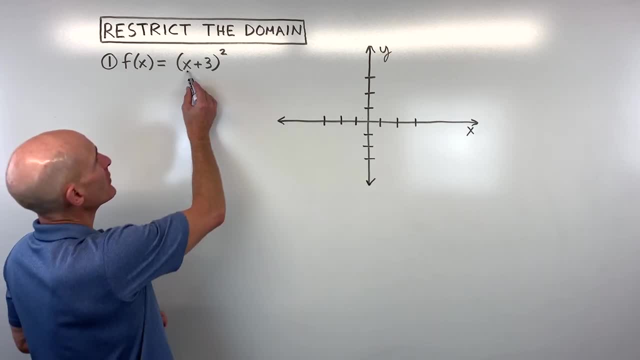 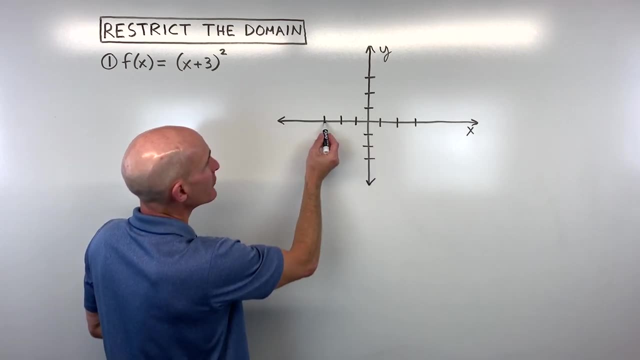 let's just graph this to get a sense of what this graph looks like. Now we know that x squared, that's a parabola shape, and the plus 3 here is going to have the opposite effect. It's going to shift the graph left- 3.. 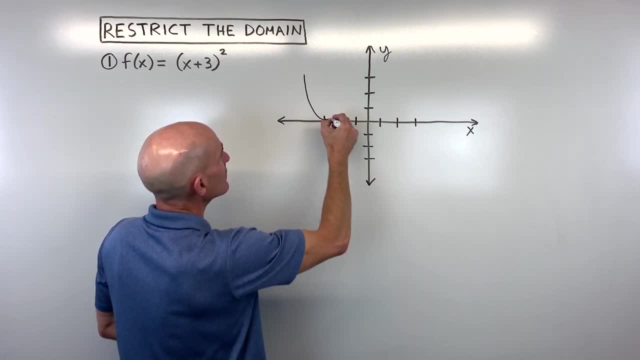 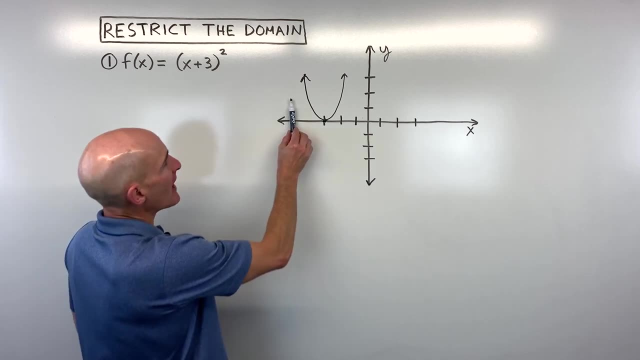 So this graph is going to look something like this, roughly Okay. now when you do the vertical line test what the vertical line test, it tests to see if this graph here is a function, meaning for every x value there's only one y value. 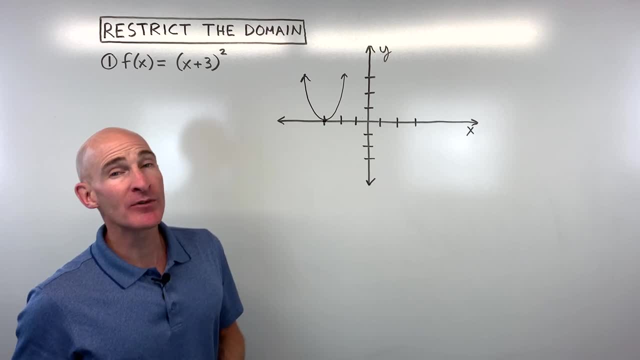 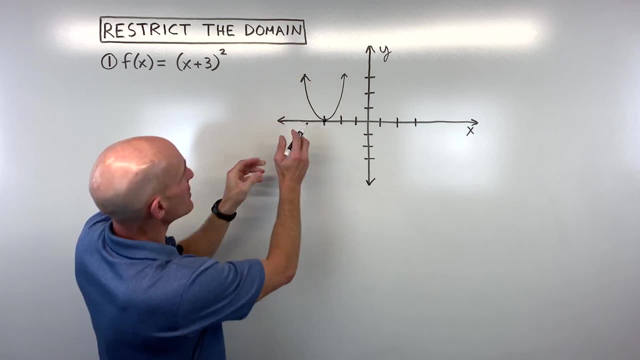 And you can see that it passes that vertical line test. But there's something called the horizontal line test, where you take a line like this and you scan up and down and you see if the graph crosses more than once, And in this case, 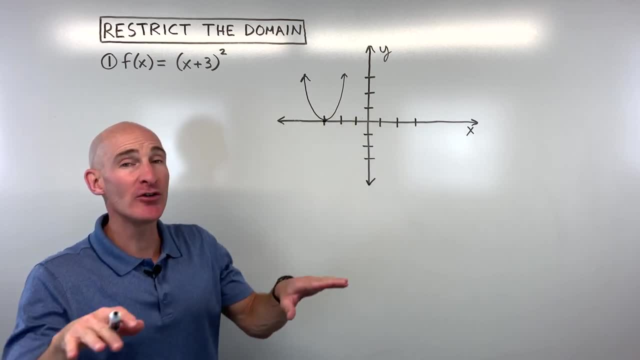 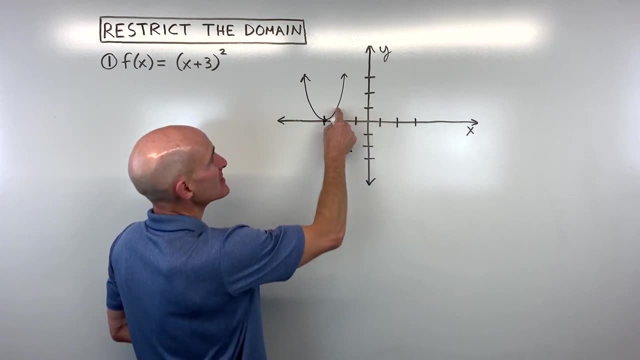 you can see that it does cross more than once, which means that it fails that horizontal line test, meaning that the inverse is not a function. So for every y value, see how there's more than one x value. So what we're going to do is we're going to restrict the domain. 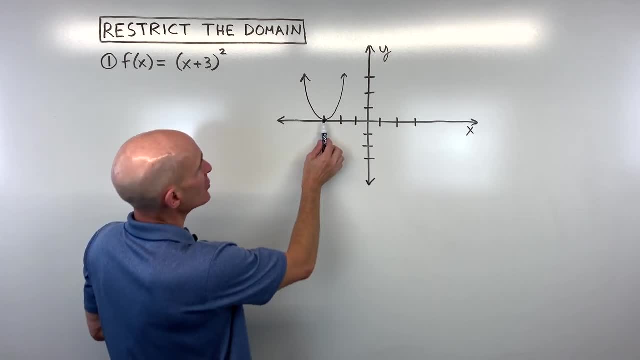 Now we have two options with this problem. We can either say that we're going to look at just this right branch of the graph, this part right here, or the left branch of the graph, because if I just look at one half of this parabola, 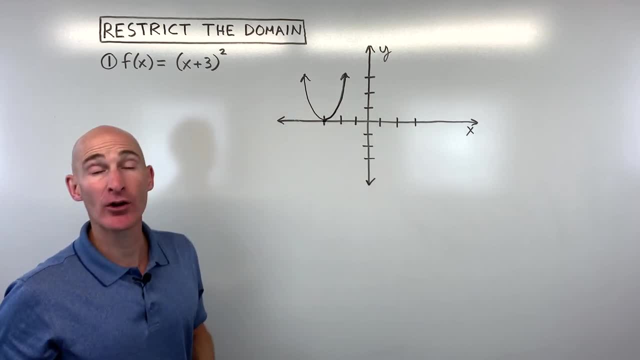 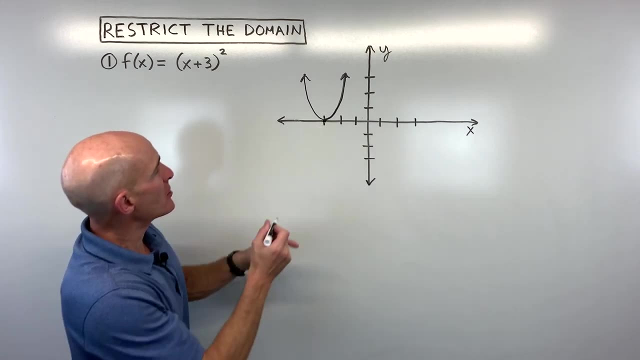 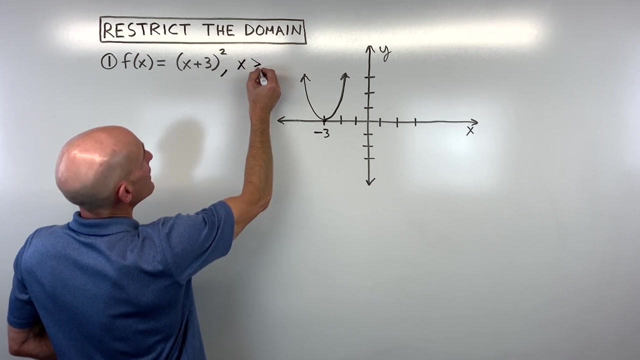 it would pass that horizontal line test, meaning the horizontal line would only cross the graph at most once. So let's do this problem two different ways, so you can see both ways. So here at negative 3, if we restrict the domain and say where x is greater than or equal to negative 3,, 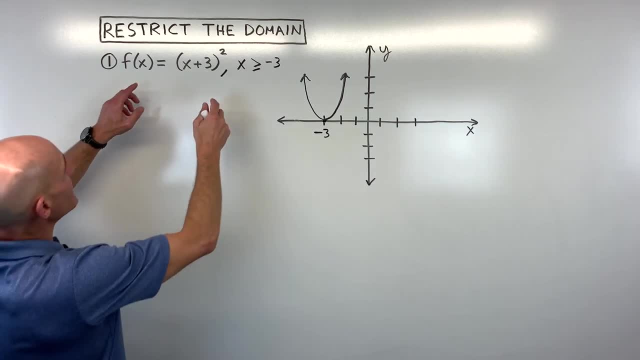 and we find the inverse. now what we're going to do is we're going to interchange the x and the y and we're going to solve for the new y. So when you think of f, of x, you can think of this as our output or our y value. 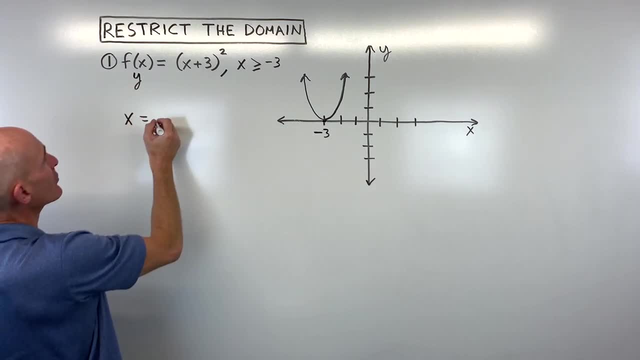 So we interchange the input and the output, or the x and the y, and then we solve for the new y. So here, what I'm going to do is I'm going to take the square root of both sides. Okay, the square, and the square root cancel. 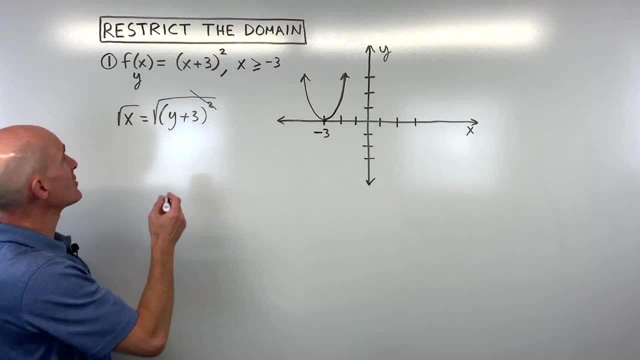 Remember, when you take the square root of both sides of the equation, you get two answers: plus or minus, Okay, positive or negative. And so now we're down to y plus 3 is equal to positive or negative. square root of x. 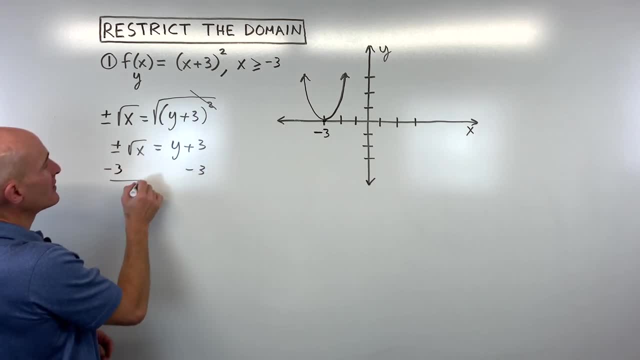 And then if I subtract 3 from both sides, this comes out to: let's see: plus or minus: square root of x minus 3 equals y, Or let's just flip it over so we can see it from a different perspective here. 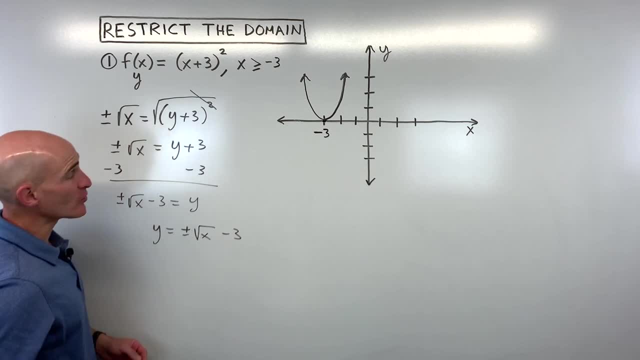 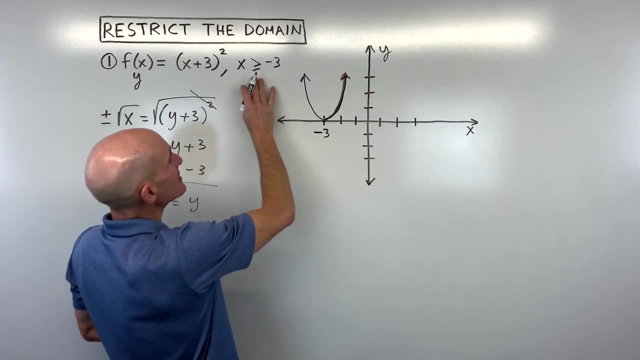 y equals plus or minus the square root of x minus 3.. Now going back to this original graph here, let me make this a little bit darker. See, we said the domain is what the x's can be. x is greater than or equal to negative 3.. 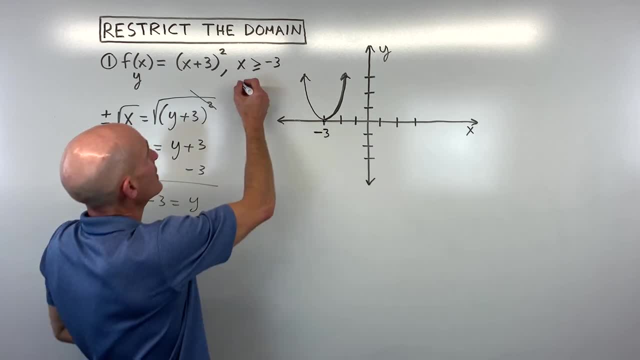 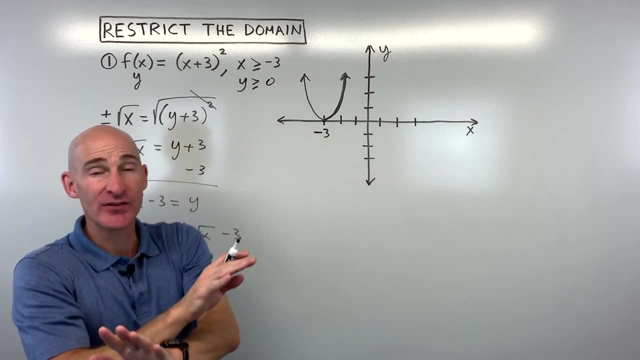 The range is what the y's can be, And here you can see that y is greater than or equal to 0.. But what happens when you interchange the x and the y? the domain and the range switch as well, because the domain is associated with the x. 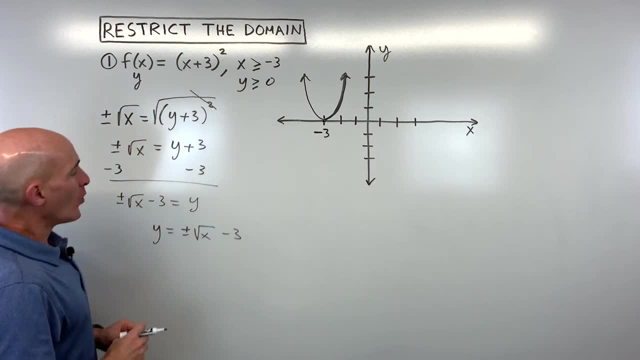 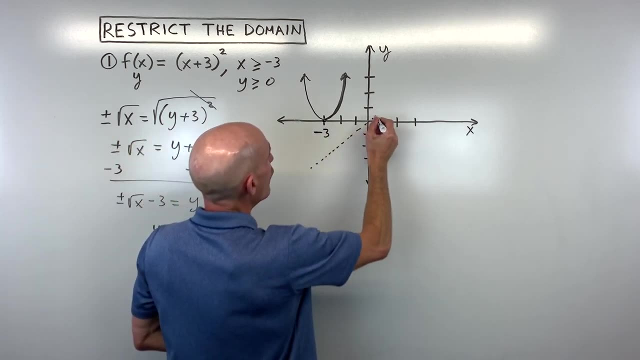 and the range is associated with the y right. So what happens here is we're going to look at this graph And when you find the inverse, you're reflecting that graph. over the line y is equal to x. That's what happens when you find the inverse. 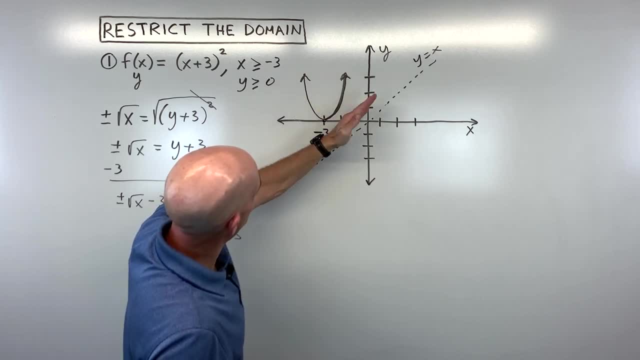 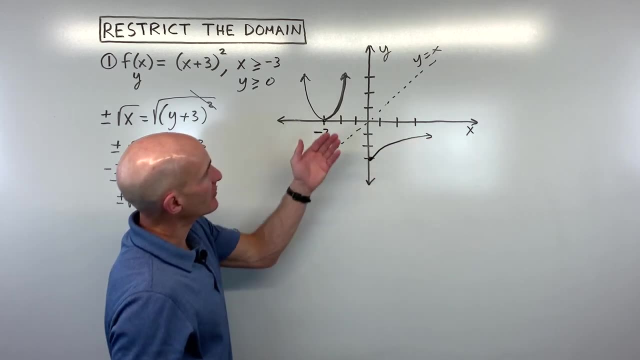 And so if you look at this branch of the, the right branch of this graph, when I fold it over this line, y equals x, we're going to get a graph that looks something. that looks like that. okay, It's just the mirror image. 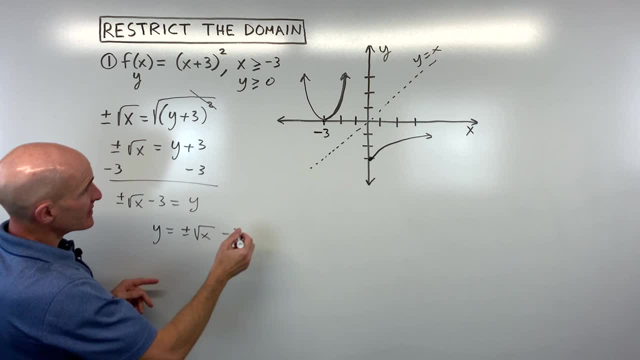 Now when you look at this here, you say, oh, okay, so that means that this is: y is equal to the positive square root of x minus 3,. okay, And you could write this in the inverse notation: f. inverse of x. 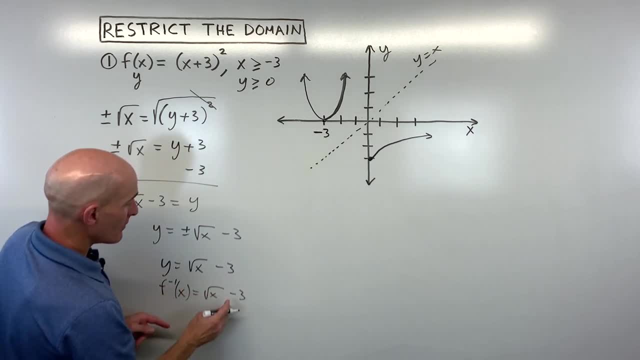 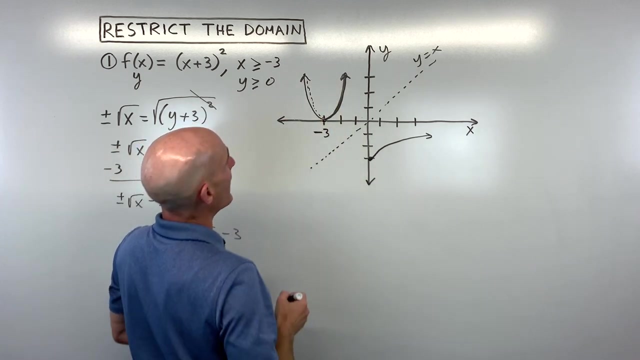 That's what this minus 1 represents. equals square root of x minus 3.. And that's this branch right here. Now, if we were to do this another way here, by looking at the left branch, okay, So let's maybe draw this as a dashed or dotted line, like that. 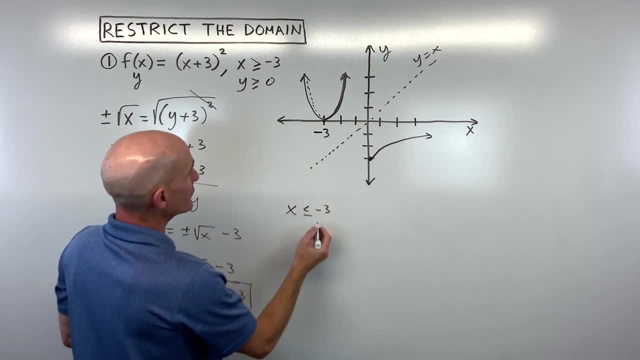 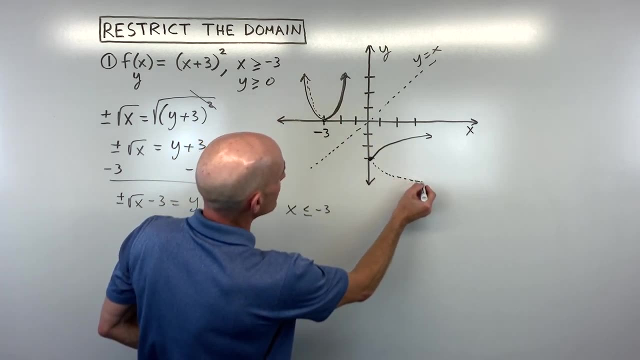 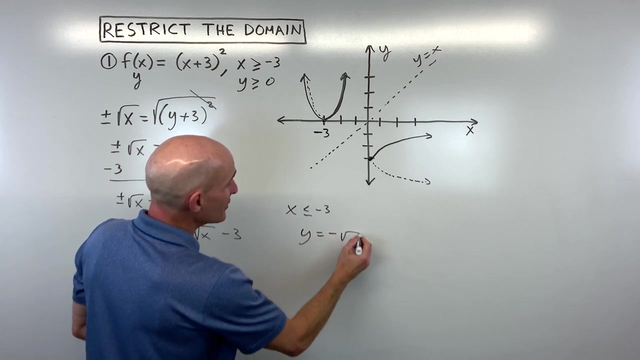 Now we're saying, okay, let's let x be less than or equal to negative 3.. When we take this dash graph and we refold it over the line y equals x, we're going to get this graph right here. Which this graph is? the graph y is equal to negative square root of x minus 3.. 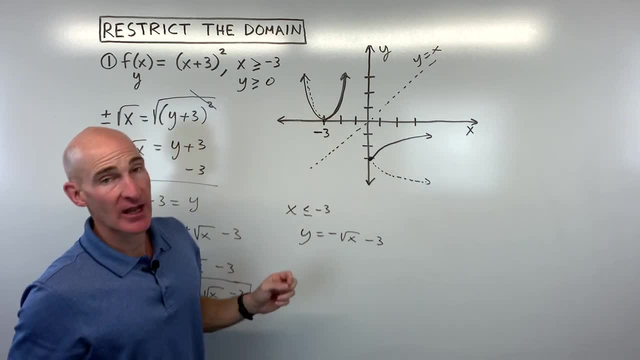 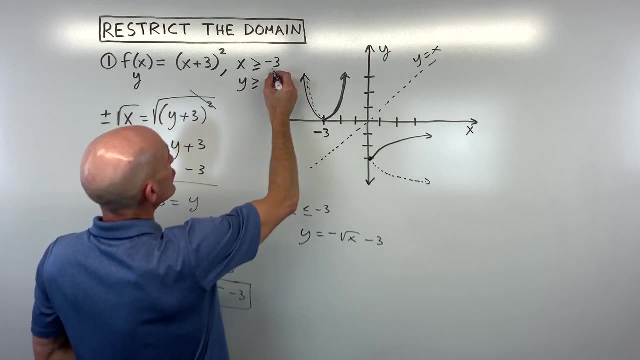 So, depending on which part of the graph that you use, you have to kind of pay attention when you find the inverse. Now what's interesting is see here: I've written this in inequality notation. Let's write it in the interval notation. 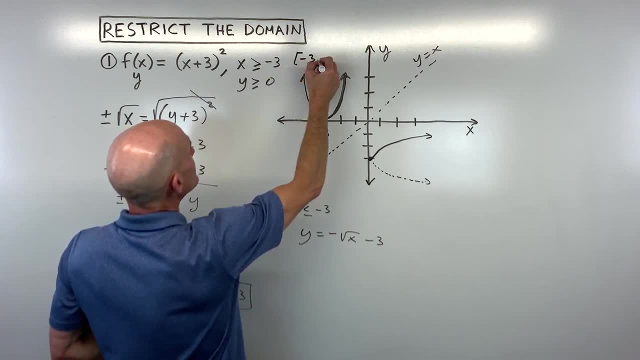 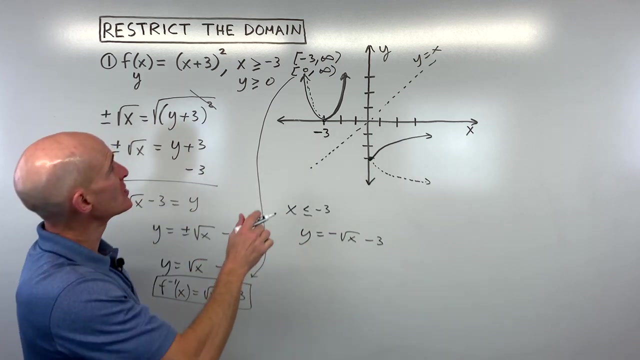 So the domain is going to be from negative 3 to infinity And the range is going to be from 0 to infinity. But what happens when we find our inverse graph? okay, over here, remember how we said: the domain and the range switch. 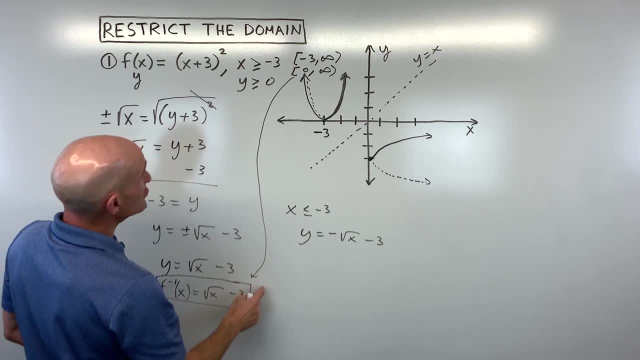 So this range here would really become the domain here, And that's going to be where x is greater than or equal to 0. Or you could say from 0 to infinity, And you can see that's what's happening right here for the domain. 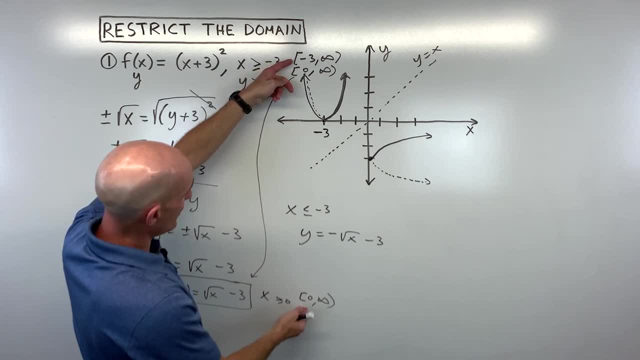 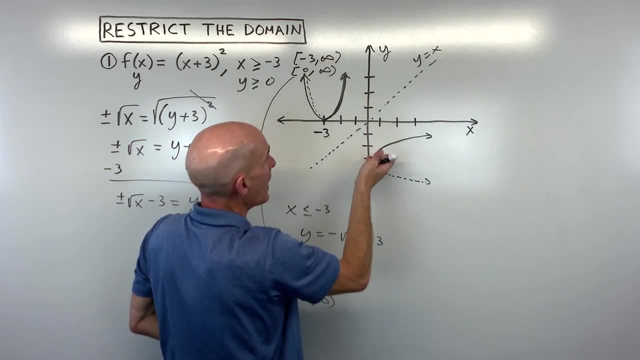 Now, as far as the range of this inverse function, the range would be negative 3.. To positive infinity, And you can see this is going from negative 3 and upward, like that. So what you can see is that if you find the domain and the range on the original graph, 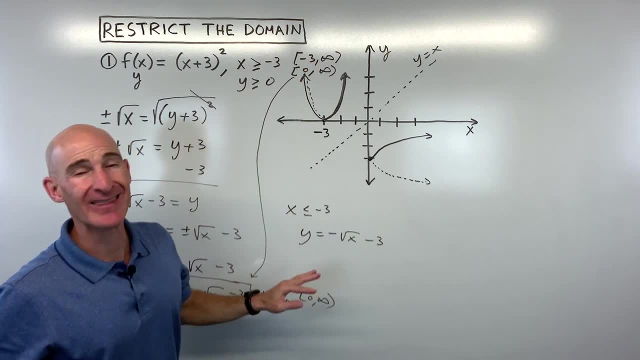 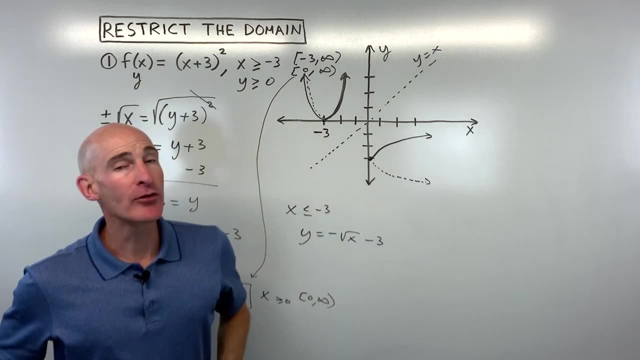 by interchanging those, you'll know what the domain and the range are on the inverse graph, And so that'll help you when you're graphing and it'll just help you when you're writing your notation. Let's take a look at another example. 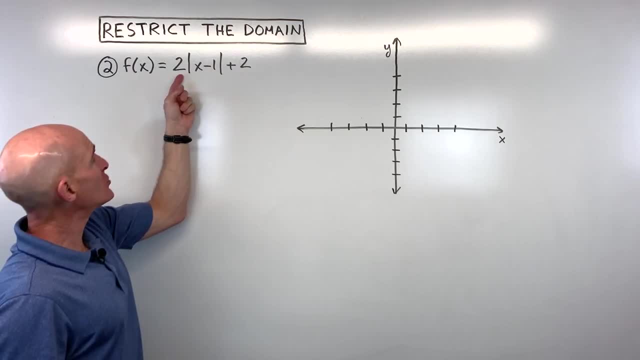 Okay, for example, number 2- now we have f of x is equal to 2 times the absolute value of x minus 1 plus 2.. Let's start off by graphing this to get a sense of what this looks like. We know that this graph is going to be going right: 1, up 2.. 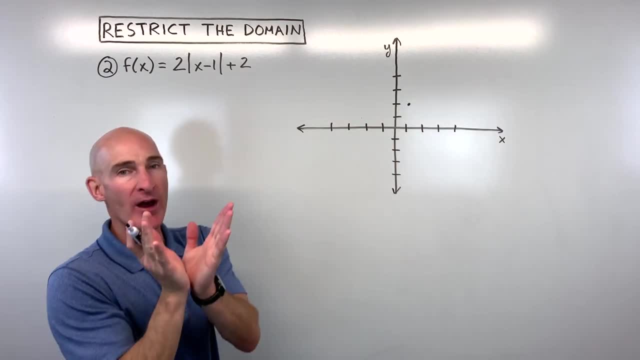 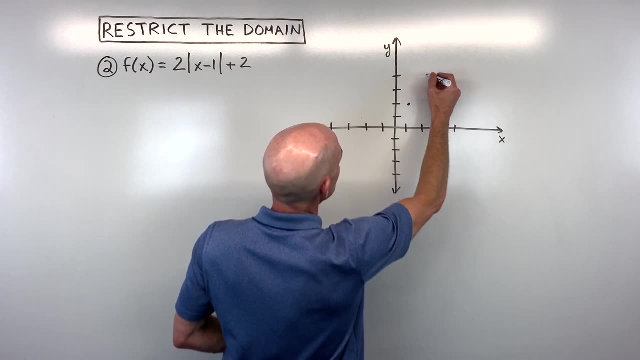 And so this is where the vertex of the absolute value graph is, And we know it's being stretched vertically by a factor of 2.. So this is going to have kind of like a slope of 2.. You're going up 2 over 1, up 2 over 1.. 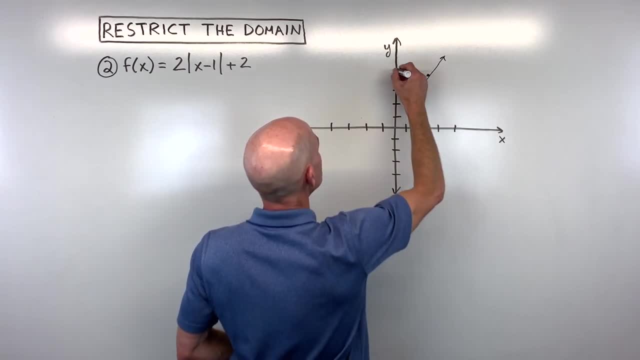 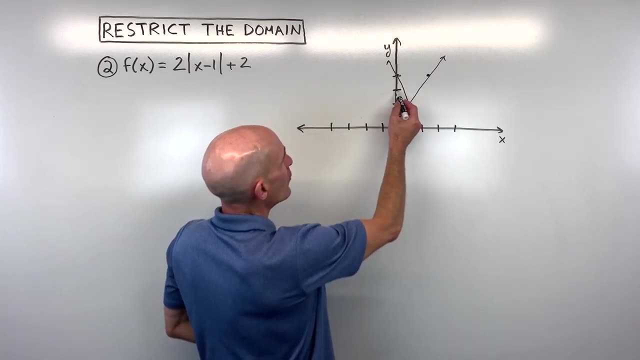 And so there's our absolute value graph. Okay, now, when we look at this, we can see that it's failing that horizontal line, That horizontal line test, right? So that tells you, for a given y value, you can see there's more than one x value. 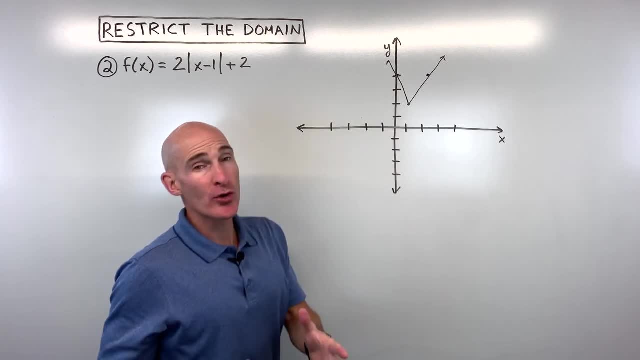 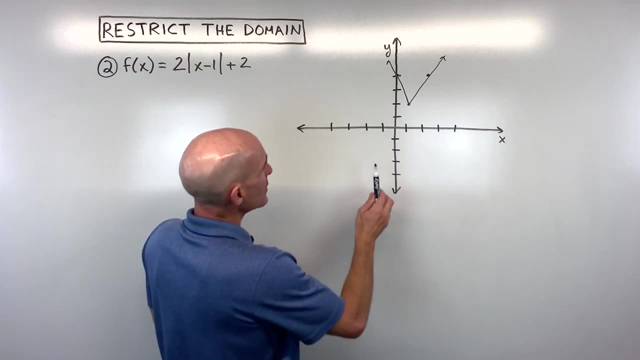 which means that the inverse is not going to be a function. So what we're going to do in order to make the inverse a function, we're going to restrict the domain, meaning what the x values can be, And so let's take a look at this right branch of the graph, right here. 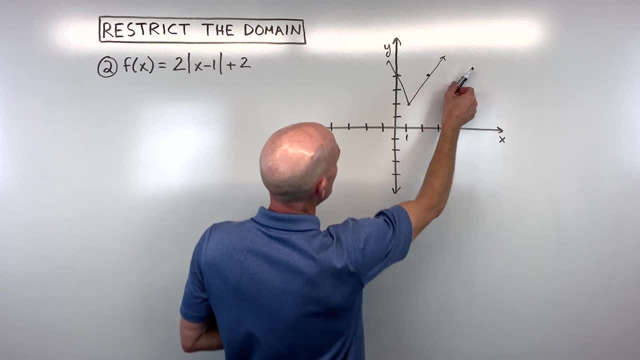 Let's see right here where x is 1.. If we just go to where it's right of 1, just this right branch. Let me make it a little bit thicker, a little bit wider here, so we can see it a little bit better. 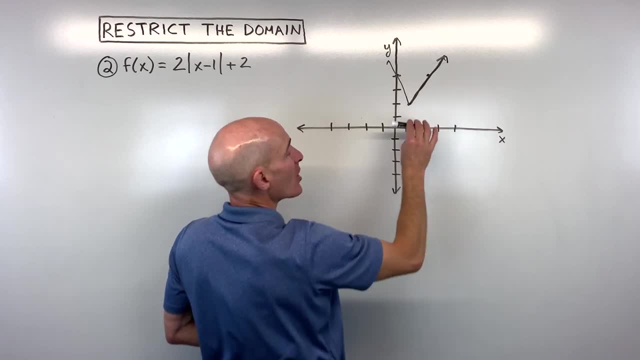 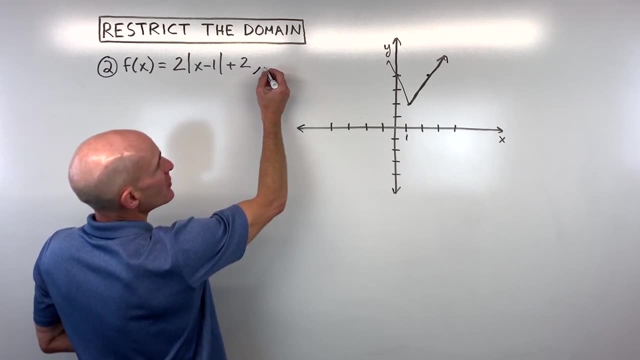 Now, when we do the horizontal line test, you can see it crosses only at most once. So that tells us that the inverse will be a function. So let's go ahead and put our restriction here. Let's say when x is greater than or equal to 1,. 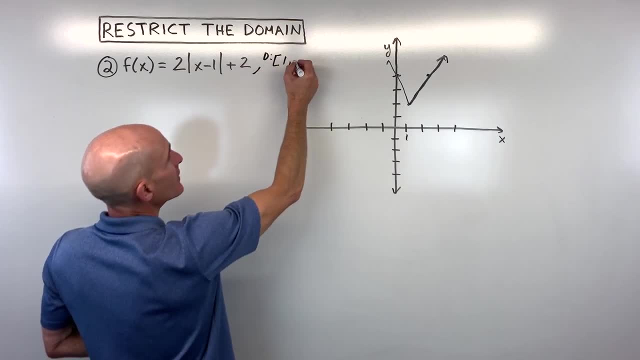 or we'll just say from. for our domain, we'll say 1 to infinity. Now the range is going to be the y values. You can see that that's going to be from 2 to infinity. Now let's go ahead and find the inverse. 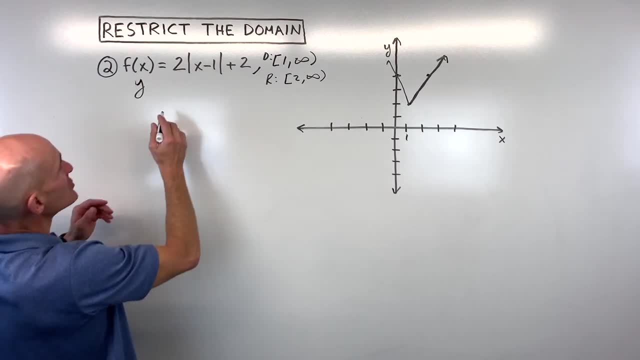 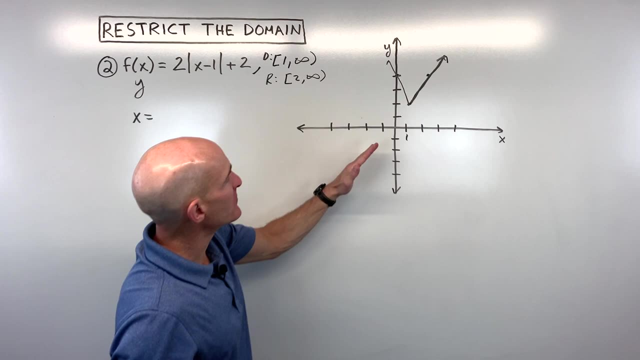 Remember, we switch the x and the y and we solve for the new y. So if I do that, we get x is equal to Now. let's take a look at this line for a moment. So this is really like a line: half of this absolute value graph. 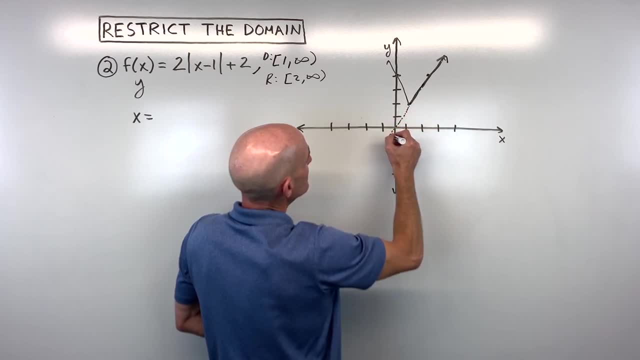 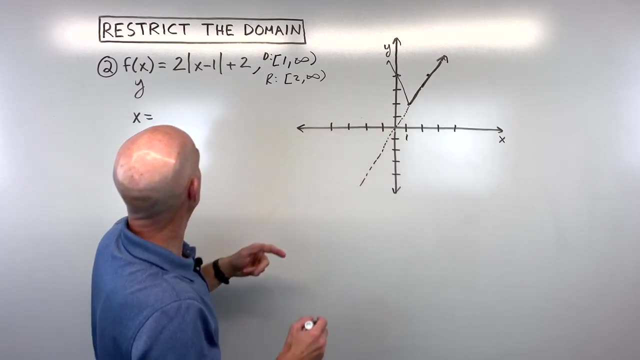 And this line you can see if I kind of continue it down like this: okay, that's our line, And so it has a slope of 2 and a y-intercept of 0. So really, the equation of this line is just: y is equal to 2x plus 0,. 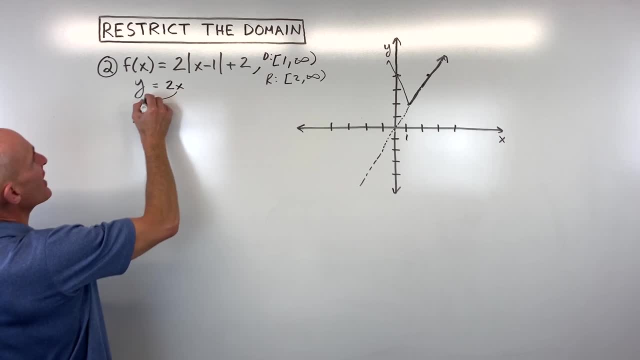 or just y equals 2x. So I'm just going to interchange the x and the y and solve for the new y. So to get this y by itself, I'm going to multiply both sides by 1 half, And so now we get 1 half. x is equal to y. 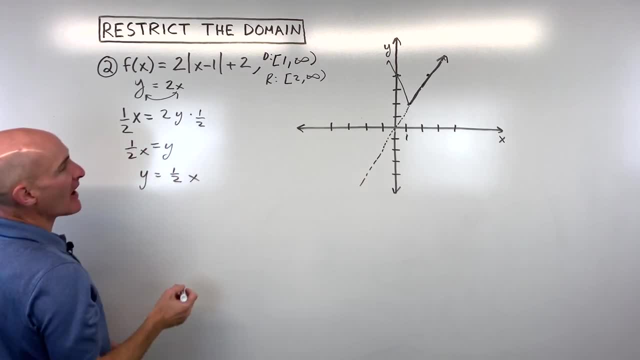 or, if I flip it, y is equal to 1 half x. Or we can write it in the inverse notation by saying: f inverse of x is equal to 1 half x. Now remember, when you find the inverse graphically, what it looks like. it's a reflection over the line y equals x. 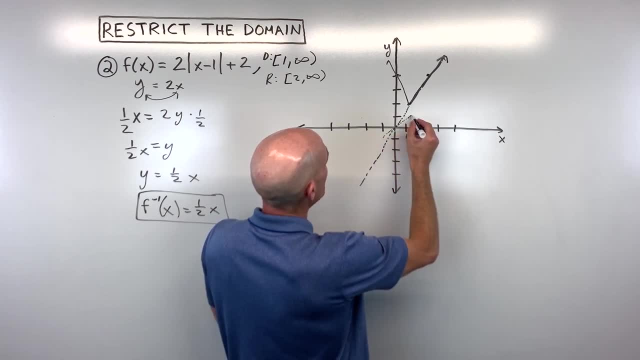 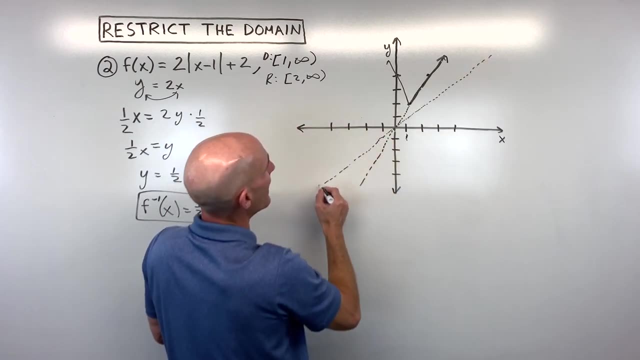 So the line y equals x is this 45 degree line. It has like a slope of 1. So I'll try to draw it accurately here for us. So it looks something like that. right, Let's label that y equals x. 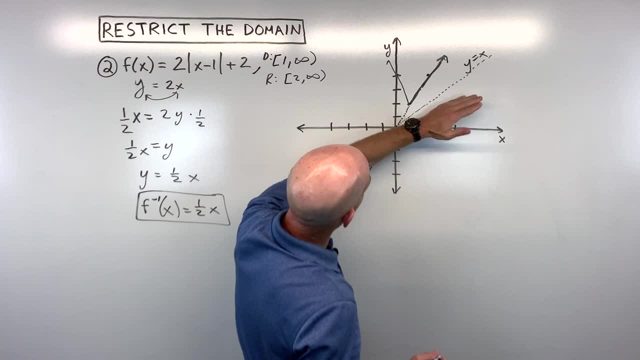 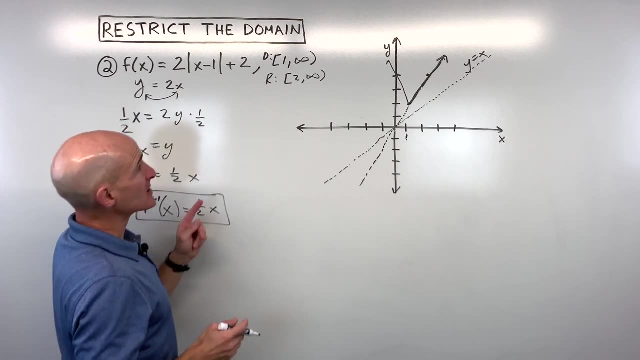 And when I fold that right branch over that graph, it's going to look something like this: right, And it's going to be: the line y equals 1 half x. But notice, the domain and the range are switching, So the range becomes the domain over here. 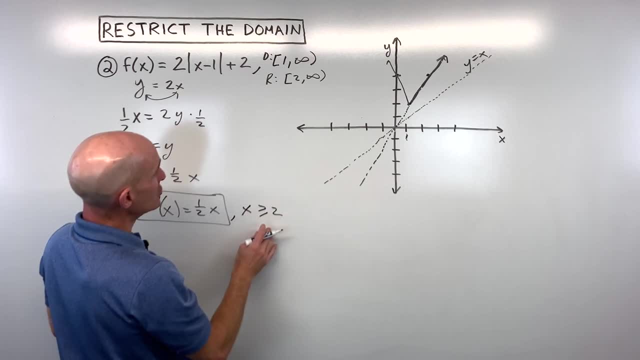 So this is going to be: x is greater than or equal to 2, or in interval notation you could say, from 2 to infinity, And the range is going to be from 1 to infinity. So basically we're graphing this line: y equals 1 half x. 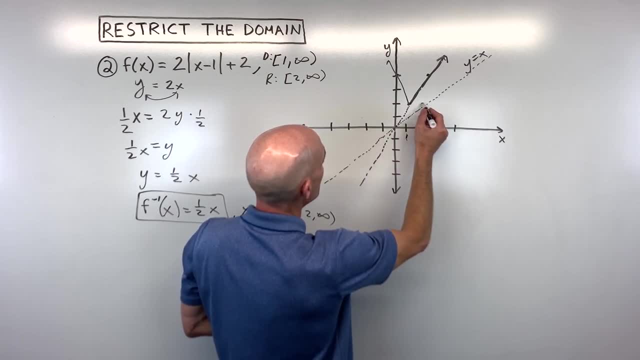 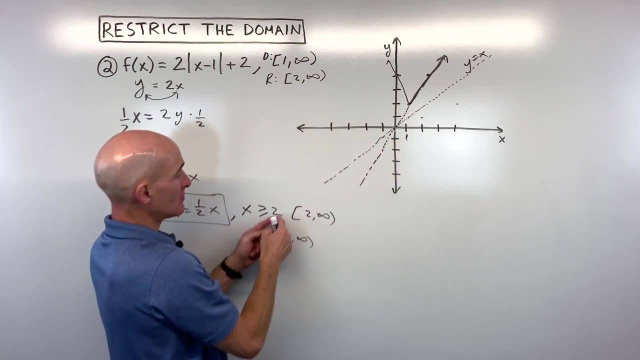 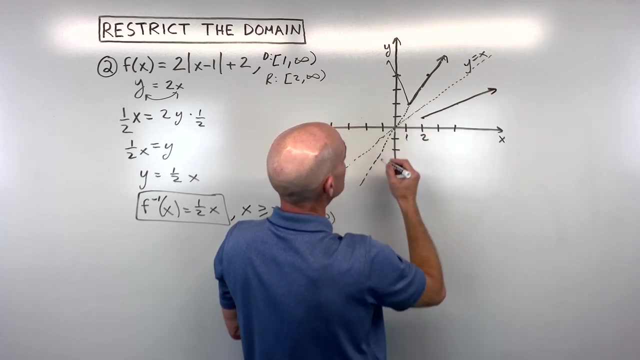 which would look like this: Rise 1, run 2,, rise 1, run 2.. But we only want the part of this line where it's greater than or equal to 2.. So from here onwards, we just want this part of the line. 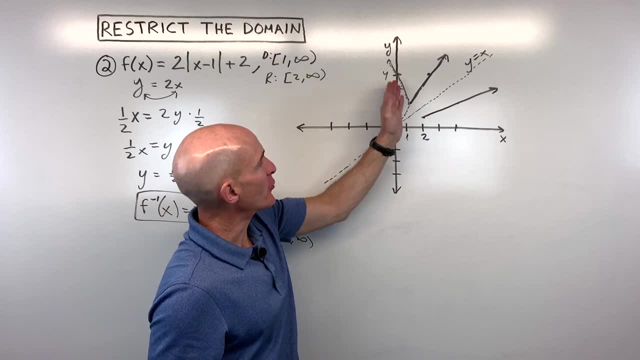 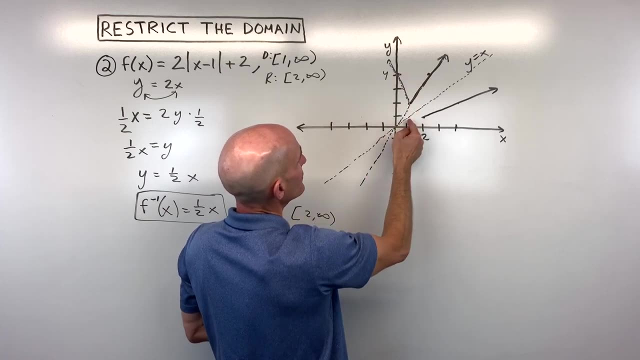 Okay now looking at the other half of the absolute value graph, the part of this graph here I've drawn as a dashed or dotted line. we're going to look at where x is less than or equal to 1, or to the left of 1. here. 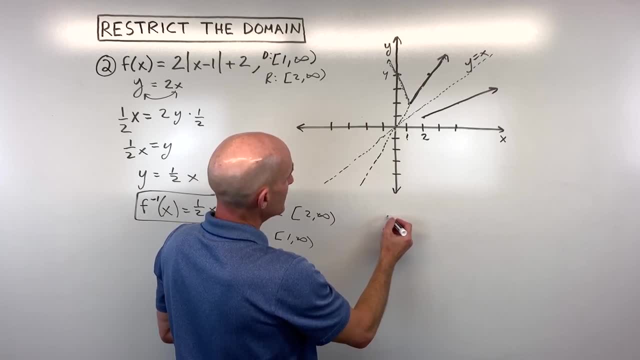 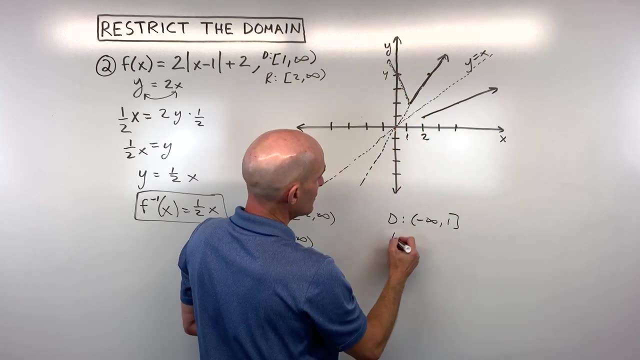 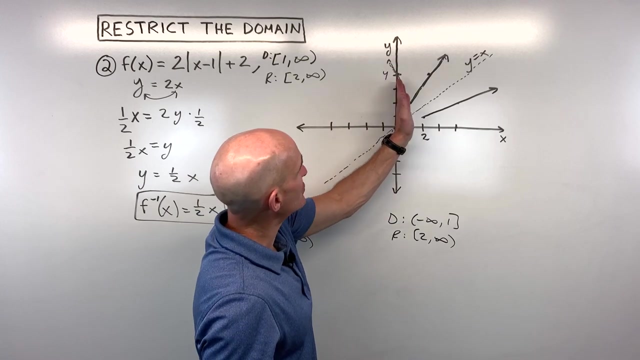 So if we do that, we're going to be looking at a domain of negative infinity to 1, and the range is still going to be from 2 to infinity To positive infinity. But when you look at this dashed or dotted line, 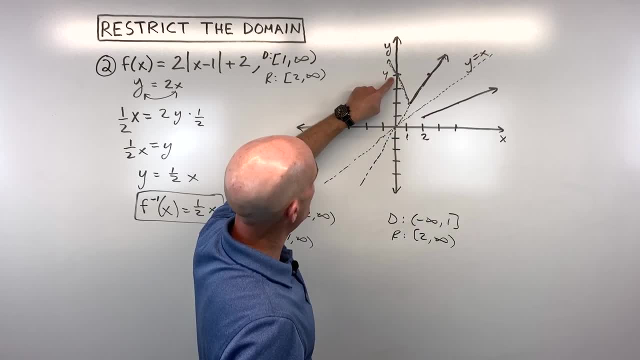 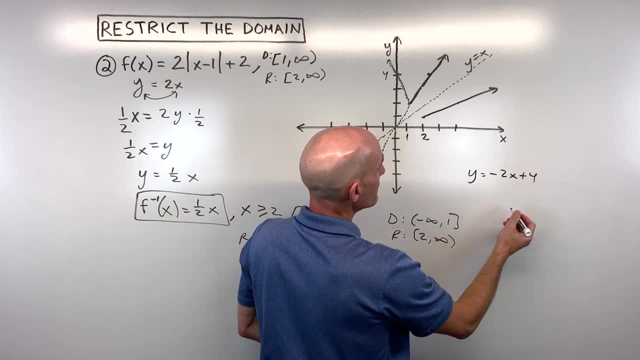 what's the equation of that line? Well, it has a y intercept of 4, and it has a slope of negative 2.. So our equation is really: y is equal to negative 2x plus 4.. To find the inverse, we interchange the x and the y. 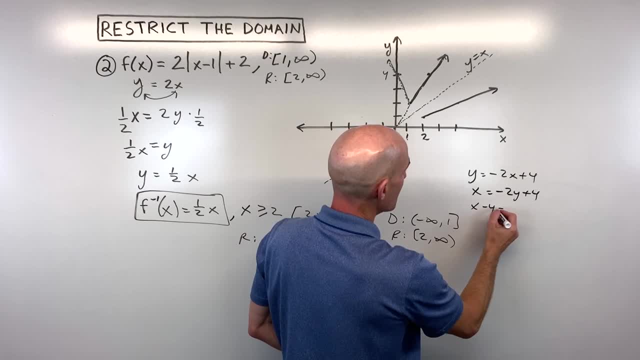 and we solve for that new y. So I'm going to subtract 4 from both sides and multiply everything by negative 1 half, So that will give us negative 1 half. x plus 2 is equal to y, or we can flip it and use the inverse notation. 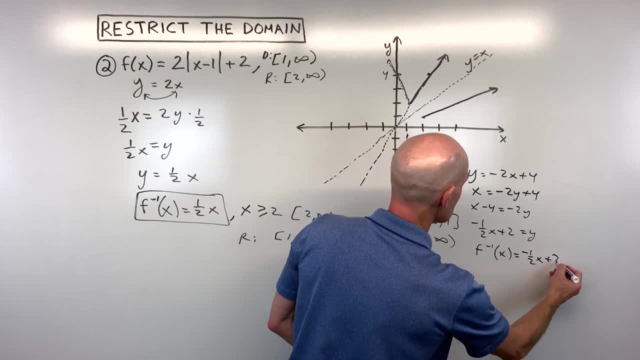 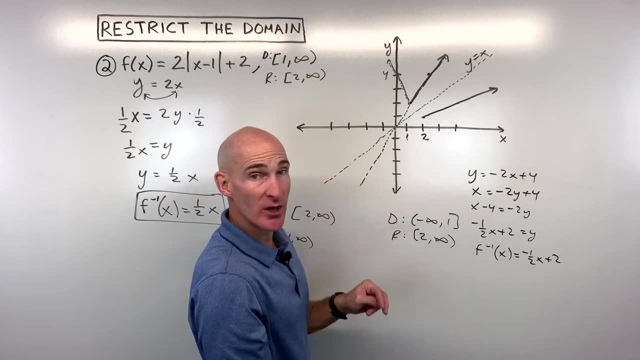 f inverse of x is equal to negative: 1 half x plus 2.. And we want to keep in mind that when we find this inverse, the domain and the range switch right. So what happens is the range actually becomes the domain of our inverse function. 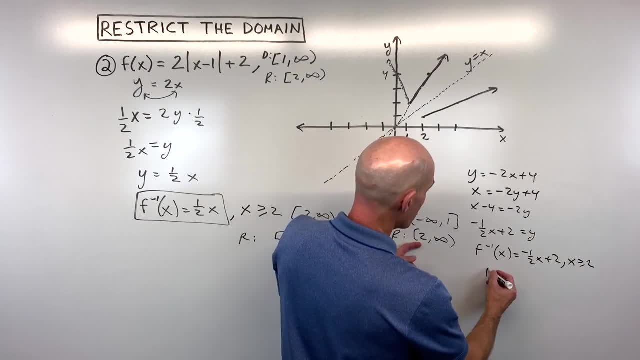 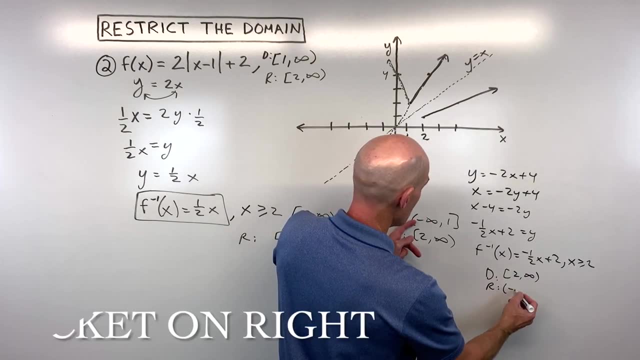 So we could say x is greater than or equal to 2, or, if you're using the interval notation, you can say from 2 to infinity and our range is going to be from negative infinity to 1.. Now, graphically, what that looks like. 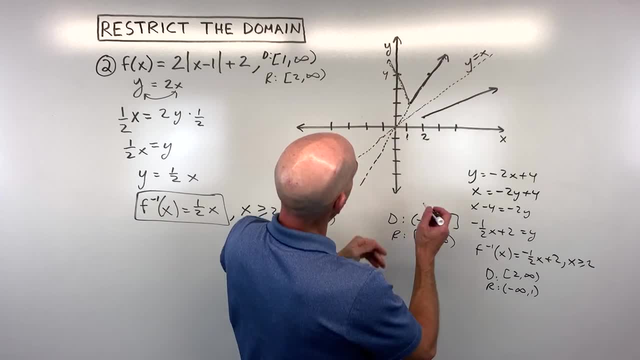 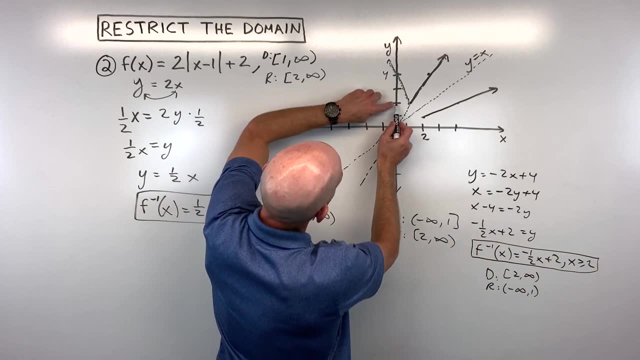 when you fold this dashed or dotted line over the line y equals x. it's going to look like this equation right here: negative 1 half, x plus 2.. Now here's the y intercept of 2, slope of negative 1 half. 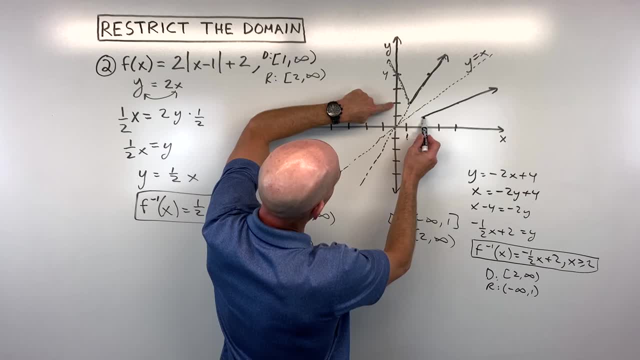 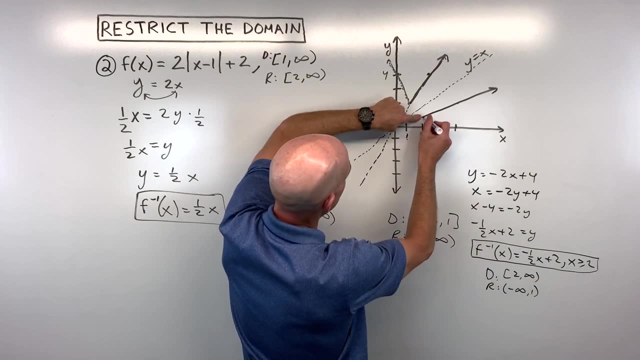 that's down 1 over 2, okay, down, 1 over 2.. What's interesting, though, is we only want to start when x is greater than or equal to 2, so we just want this part of the graph right here. 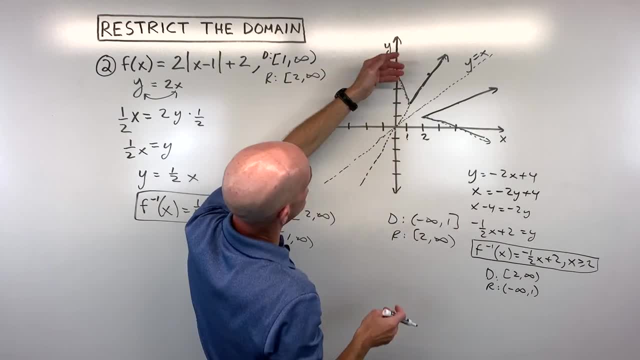 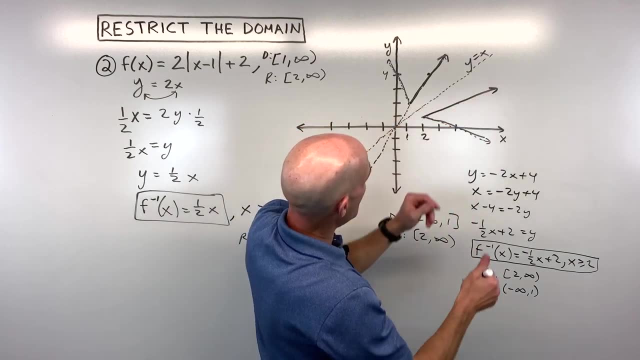 I should have drawn that as a dashed or dotted line, just to show you that it matches up with this dashed or dotted line. So you can see, if we were to take this whole absolute value graph and reflect it, we would get this v-shaped graph on its side. 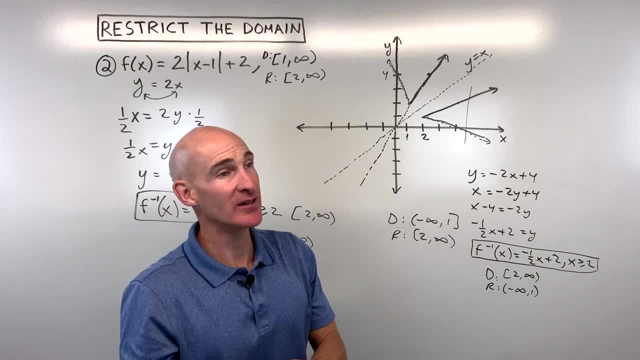 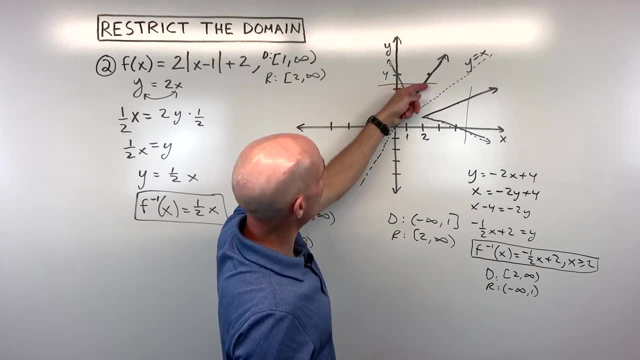 and it would fail the vertical line test, meaning that you know that this is not a function, What the horizontal line test says before you do that. if you do the horizontal line test, if it crosses more than once, then without having to graph this, 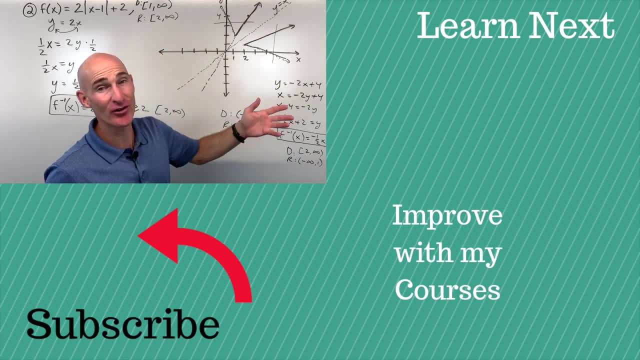 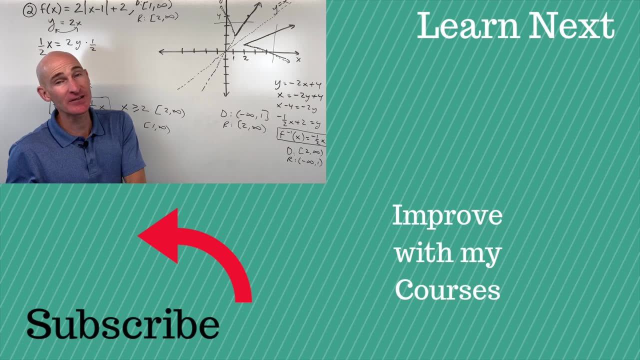 you can see it's going to pass or fail the vertical line test, So it's just a shortcut technique, but here what we're talking about is how to restrict that domain so that the inverse is a function. If you want to see more examples, 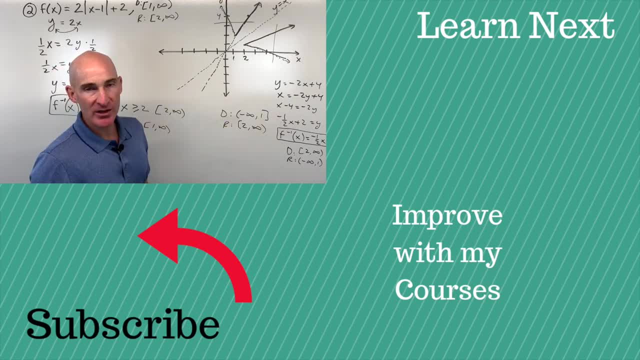 follow me to another video I did on this topic right there and we'll get some more practice. I'll see you over in that video.